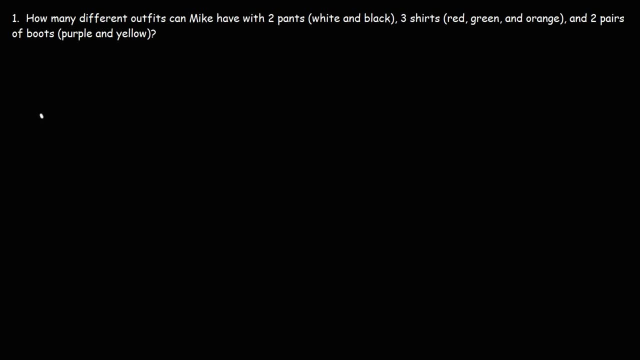 he has two pants that he will wear Either white or black. Now for a second choice. he has three shirts that he can choose from. I'm gonna color-code this so he could choose a red shirt, he could choose a green shirt, or he can choose a. 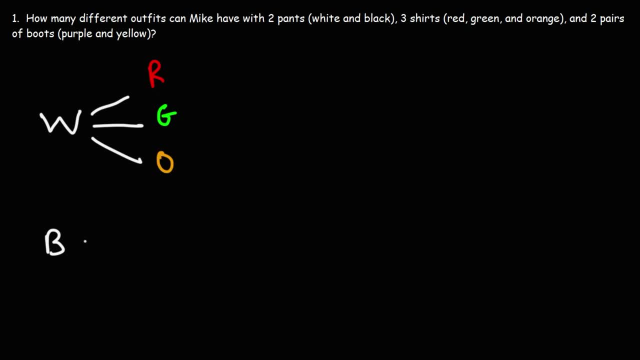 an orange shirt, and the same is true if he were to wear a pair, if he were to wear black pants. he can still pair that up with a red shirt, a green shirt or an orange shirt. now, for his next joints will be what color boots he's gonna wear. and there's 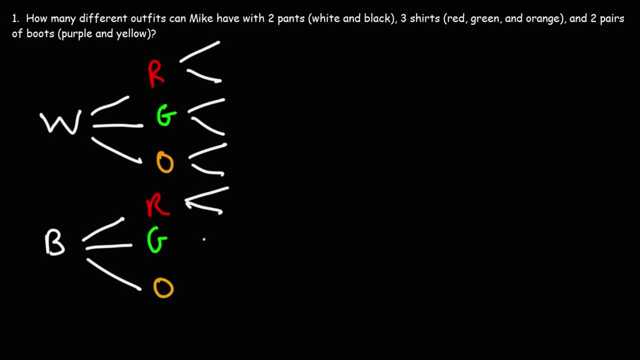 only two options here: purple or yellow. now, if we follow the tree diagram, we can get all the different possible outcomes. he could wear a white shirt- I mean a white pants, a red shirt and purple boots, so that's going to be WRP. or he could wear a white shirt. 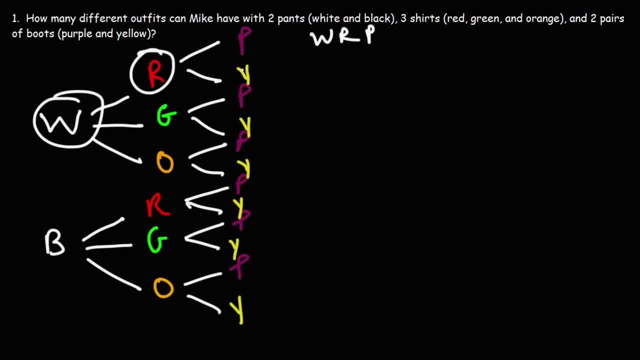 I mean, I keep messing that up- white pants, a red shirt or yellow boots, which will be a weird looking outfit, but for the sake of this problem, we'll work with it. the next option could be WGP or WGY. next is WOP and WOY. now. 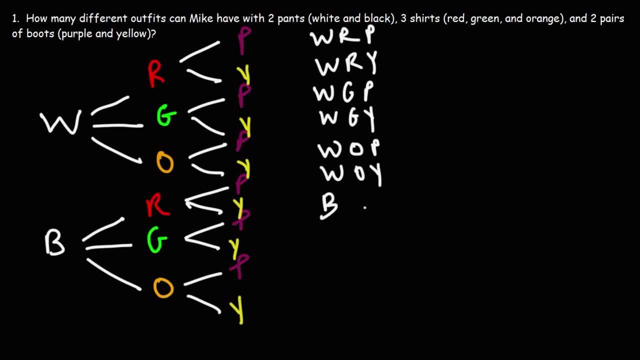 you can also choose black pants, a red shirt and purple boots, or we can have BRY. next we could have BGY- I mean BGP, let's not skip that one- you and then BGY, and then we can have BOP and BOY. so notice that what we have is a. 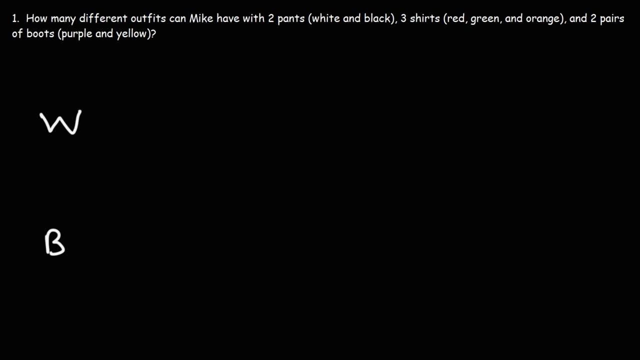 Now for a second choice. he has three shirts that he can choose from. I'm gonna color code this So he could choose a red shirt, he could choose a green shirt, or he can choose a gray shirt or a white shirt. Then he has some colors to choose from, If you. 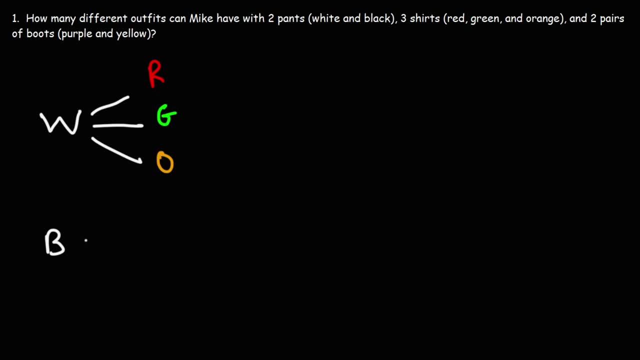 choose an orange shirt, And the same is true if he were to wear black pants. He can still pair that up with a red shirt, a green shirt or an orange shirt. Now for his next joints will be what color boots he's going to wear, And there's only two options here. 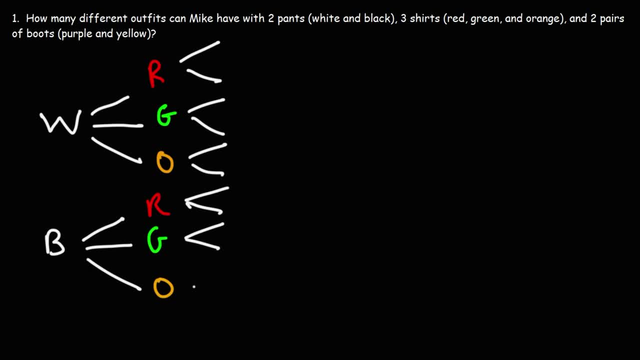 Purple or yellow. Now, if we follow the tree diagram, we can get all the different possible outcomes. He could wear a white shirt, I mean a white pants, a red shirt and purple boots, So that's going to be WRP. Or he could wear a white shirt. 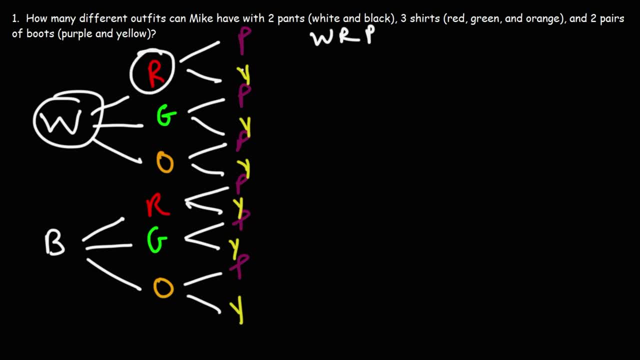 I mean, I keep messing that up- white pants, a red shirt or yellow boots, which will be a weird looking outfit, But for the sake of this problem, we'll work with it. The next option could be WGP or WGY. Next is WOP and WOY. Now you can also choose. 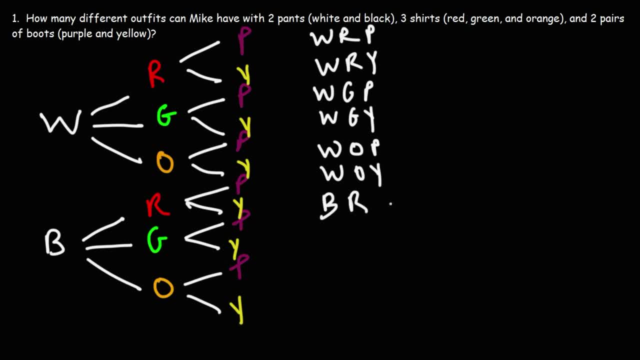 black pants, a red shirt and purple boots, Or we can have BRY. Next we could have BGY- I mean BGP, Let's not skip that one- And then BGY, And then we can have BOP and BOY. So notice that what we have is a total of 12 possible outcomes. 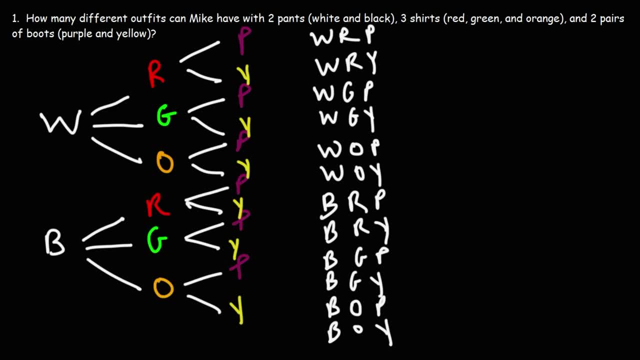 total of 12 possible outcomes. those are the different outfits that he can wear, and that's how the fundamental counting principle works. all we do is simply multiply the number of outcomes that can occur for each event or each choice that he's going to make. so for the first choice he has, 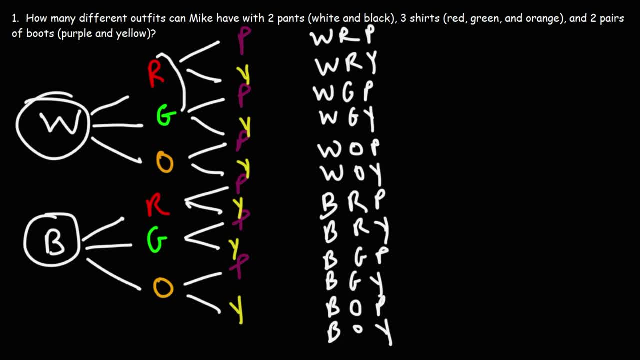 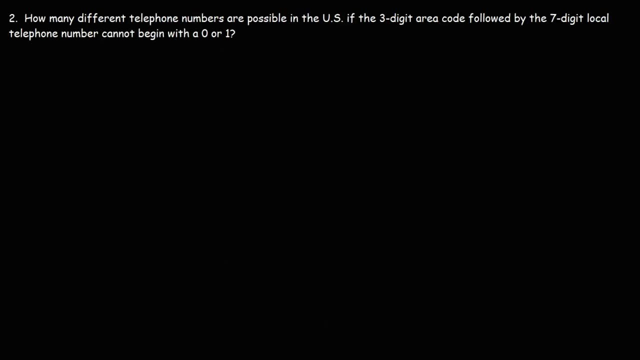 there's two possible outcomes. for the second choice there's three possible outcomes and for the third choice two. so two times three times two gives us the twelve possible outcomes that we see for the entire situation. now let's move on to the second problem: how many different telephone numbers are possible in the 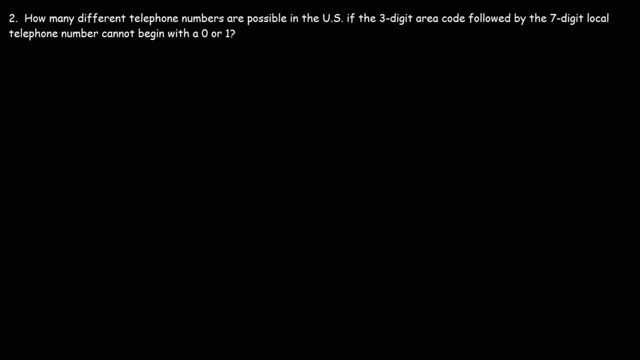 us if the three-digit area code, followed by the seven digit local telephone number, cannot begin with a zero or one. so here's an example of a telephone number. let's say three, five, seven, four, eight, six, one, two, seven, nine. so that's a typical US telephone number. so this is the three. 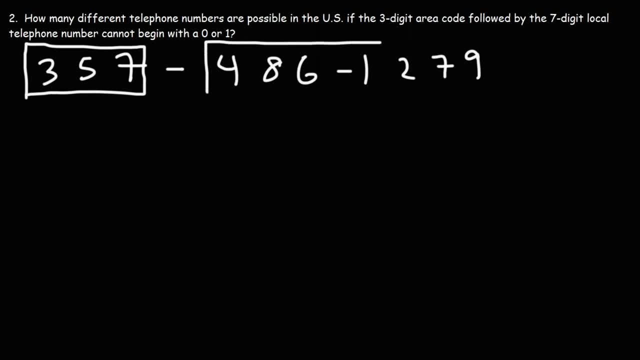 digit area code, and what we have here is the seven digit local telephone number. so we can't have a zero or one in those two spots. knowing that, how can we determine how many different telephone numbers are possible in the US? so let's start with the first digit. 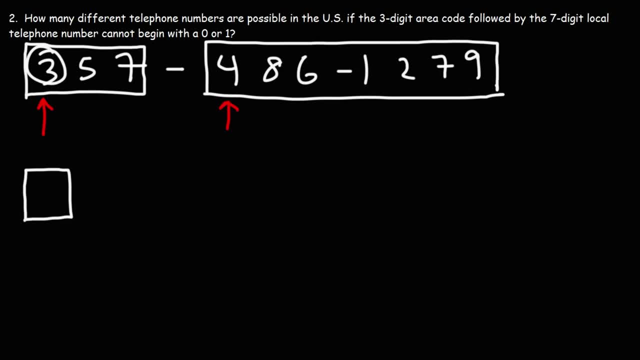 so we have the numbers: 0, 1, 2, 3, 4, 5, 6, 7, 8, 9. that's 10 possible numbers. but we can't have a zero or one. so we have eight possible choices for the first spot. now for the second spot. we can have any number from 0 to 9, so that's 10. 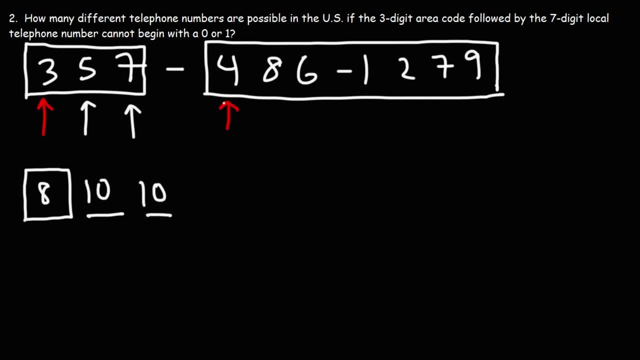 possibilities, and the same is true for the third spot. now, for this spot, we can have a zero or one, so that's going to be 8 possibilities. Everything else, we can have all numbers from 0 to 9, so that's going to be 10 possibilities. 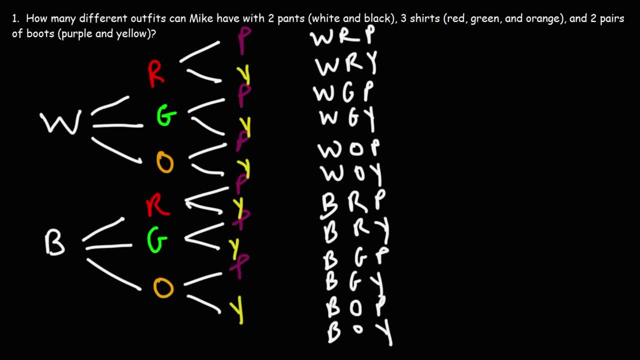 Those are the different outfits that he can wear, And that's how the fundamental counting principle works. All we do is simply multiply the number of outcomes that can occur for each event or each choice that he's going to make. So for the first choice he has, there's two possible outcomes. 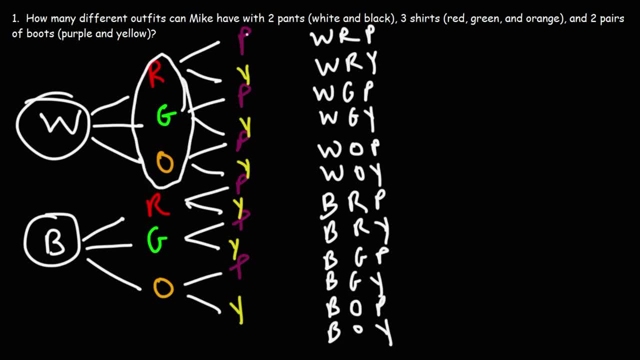 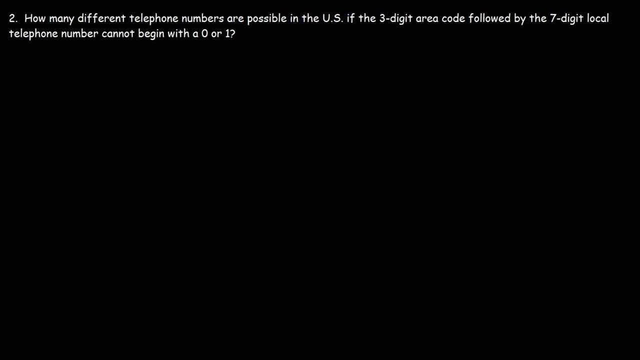 For the second choice there's three possible outcomes, and for the third choice two. So 2 times 3 times 2 gives us the 12 possible outcomes that we see for the entire situation. Now let's move on to the second problem: How many different telephone numbers? 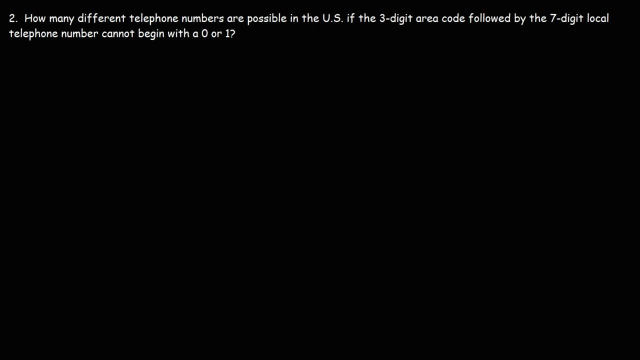 are possible in the US. if the three-digit area code followed by the seven-digit local сказать is 7? local telephone number cannot begin with a zero or one. so here's an example of a telephone number. let's say three, five, seven, four, eight, six, one, two, seven, nine. 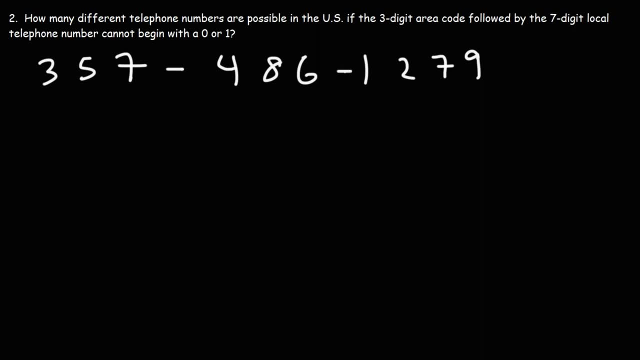 so that's a typical US telephone number. so this is the three digit area code, and what we have here is the seven digit local telephone number. so we can't have a zero or one in those two spots. knowing that, how can we determine how many different telephone numbers are? 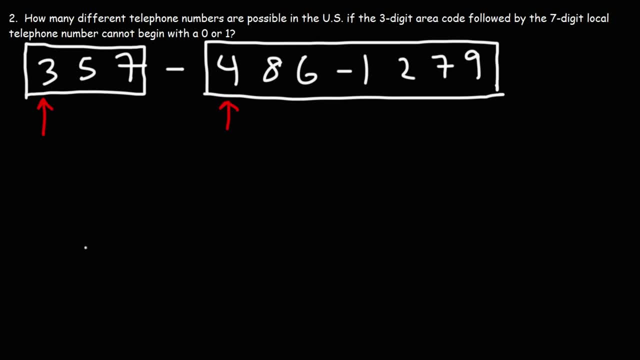 possible in the US. so let's start with the first digit. so we have the number zero, one, two, three, four, five, six, seven, eight, nine. that's ten possible numbers, but we can't have a zero or one. so we have eight possible choices for the first spot. now for the second spot. we can have any number from zero to nine. so 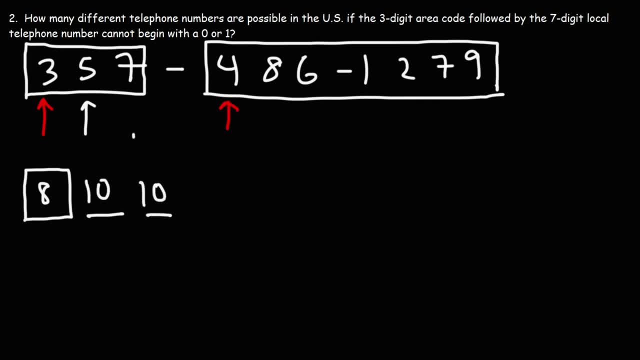 that's ten possibilities. and the same is true for the third spot. now for this spot, we can have a zero or one, so that's going to be eight possibilities. everything else, we can have all numbers from zero to nine, so that's going to be ten possibilities. 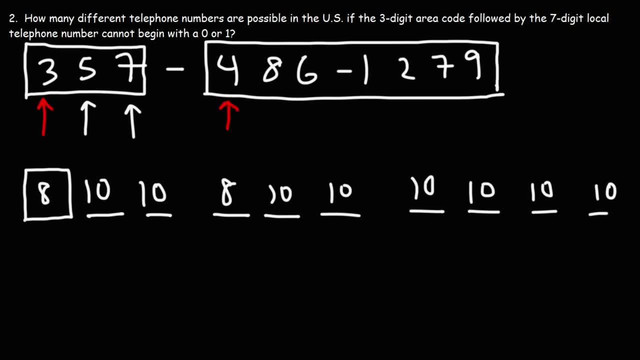 so now we need to do the math. we're going to multiply 8 by 10 by 10 by 8 by 10 by 10 and by another four tenths. so we're multiplying two eighths, that's eight squared, and we're multiplying that by eight. 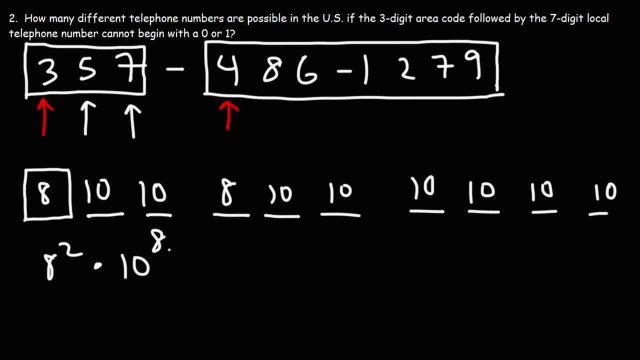 tens. so that's 10 to the eighth power. 8 squared is 64, and this is going to be times 10 to the 8. now let's put this in scientific notation: 64 is 6.4 times 10. 10 is the same as 10 to the 1, so when we multiply these two, we can add 1 and 8. 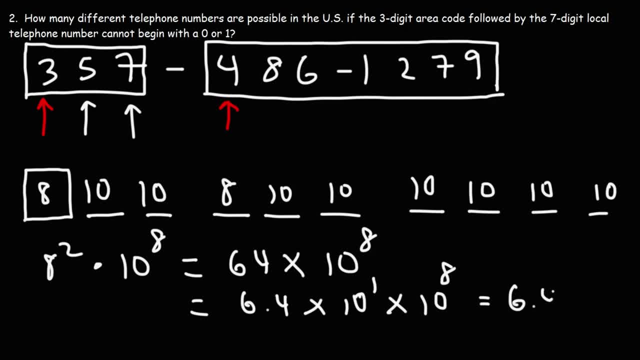 which will give us 9, so our answer is 6.4 times 10, times 10 to 9. 10 to 9 is a billion, so our final answer is 6.4 billion, which you can write it like this if you want: 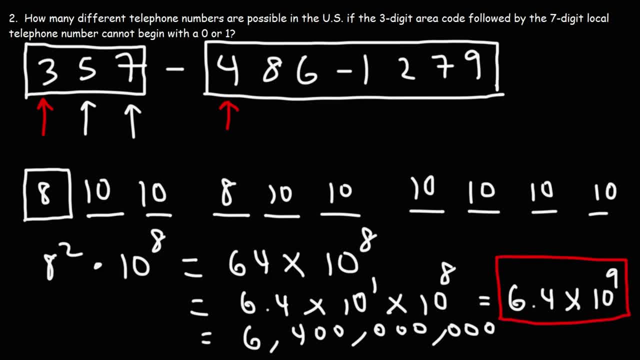 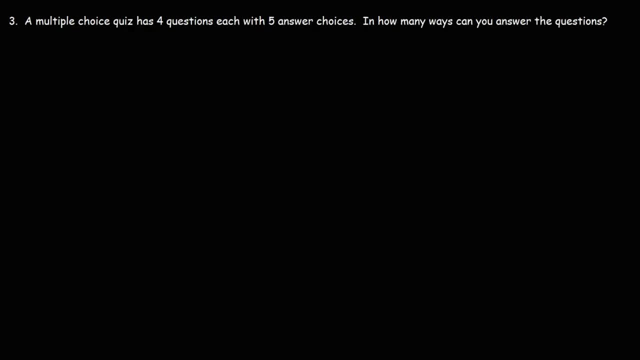 so that's how many different telephone numbers that are possible in the US with the restrictions that we can have a zero or one for the first number for the area code and the first number for the local telephone numbers. so that's how many different info we can draw. there are a lot of situations where, if we let each 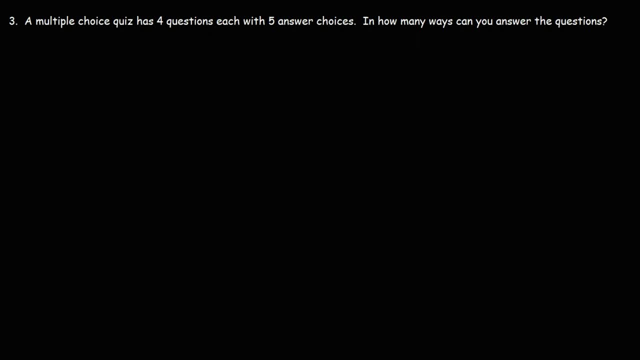 question on that nossosла. seven characters cross the, the. instead of trying to sync, byoss the local telephone number. for the sake of practice, let's work on one more question. a multiple-choice quiz has four questions each with five answer choices. and how many ways can you answer? 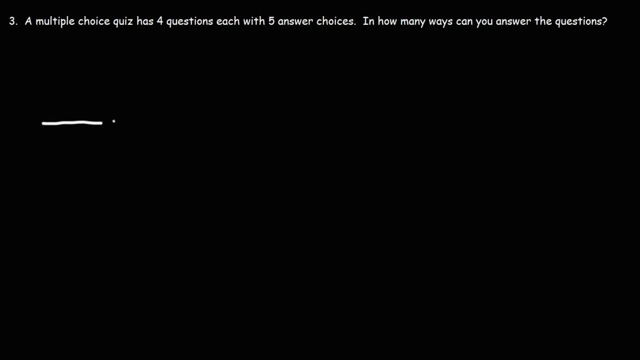 the questions. so let's say this is the first test question, this one's gonna be the second, this is the third, that's the fourth, so this situation has four events. in the first event, or the first test question, you have five answer answer choices likely A, B, C, D, E. For the next question, you also have five answer choices. 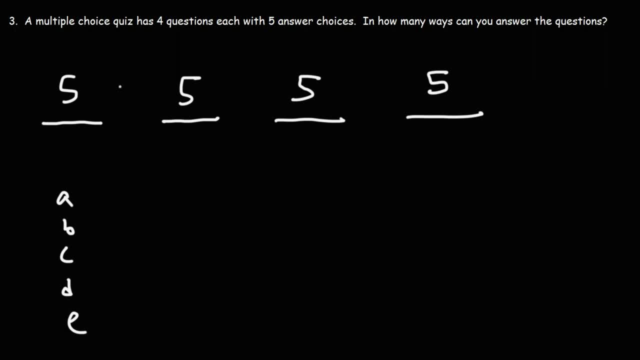 and the same is true for the third and the fourth question. So you have five possible outcomes for each event and you have four events. so this is going to be five to the fourth power, or five times five times five times five. Five times five is twenty-five and twenty-five times twenty-five. 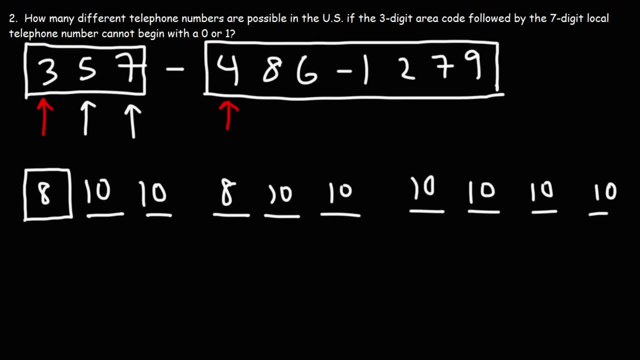 So now we need to do the math. We're going to multiply 8 by 10 by 10 by 8 by 10 by 10 and by another 4 tenths. So we're multiplying 2 eighths, that's 8 squared. 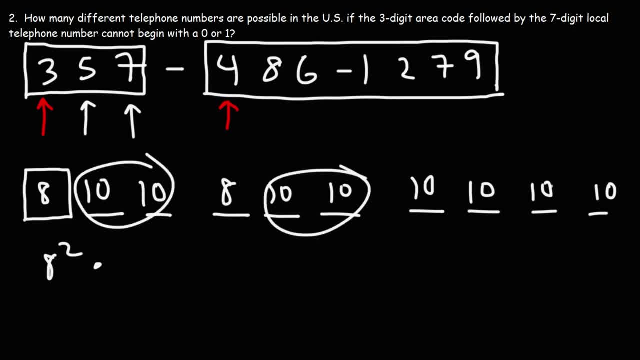 and we're multiplying that by 8 tenths. so that's 10 to the 8th. power 8 squared is 64, and this is going to be times 10 to the 8.. Now let's put this in scientific notation. 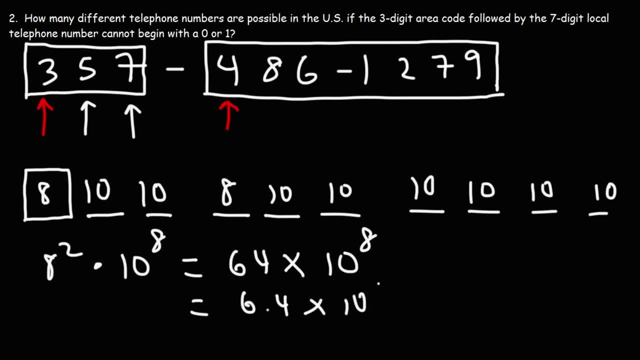 64 is 6.4 times 10.. 10 is the same as 10 to the 1,, so when we multiply these two, we can add 1 and 8. Which will give us 9.. So our answer is 6.4. 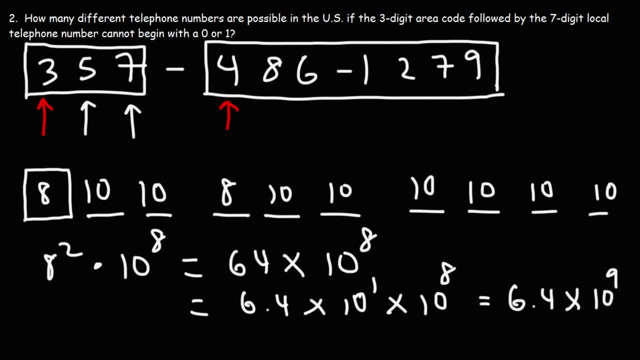 times 10 to the 9.. 10 to the 9 is a billion, So our final answer is 6.4 billion, Which you can write it like this if you want. So that's how many different telephone numbers that are possible in the US with. 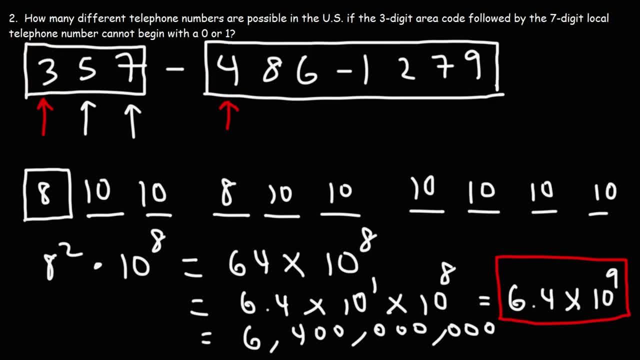 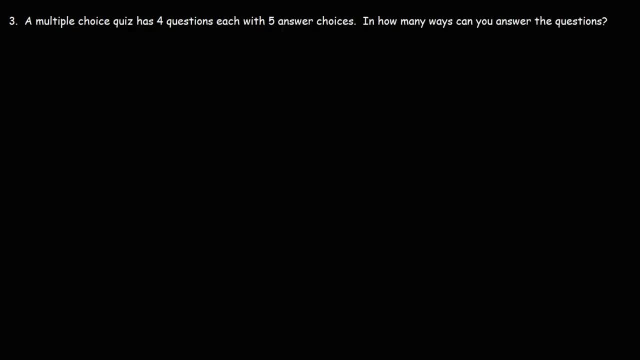 the restrictions that we can have a 0 or a 1 for The first number for the area code and the first number for the local telephone number. For the sake of practice, let's work on one more question. A multiple choice quiz has four questions each with. 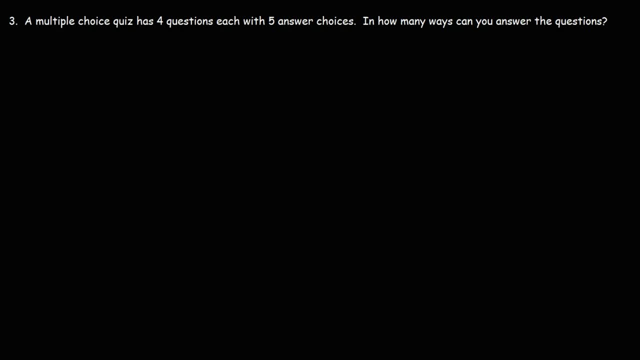 five answer choices. In how many ways can you answer the questions? So let's say this is the first test question, This one's going to be the second, This is the third, That's the fourth, So this situation has four events. In the first event, 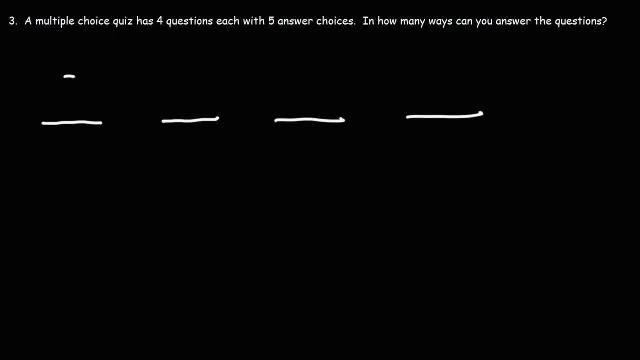 or the first test we're going to have a 4.4 billion. In the first test question you have five answer choices, likely A, B, C, D, E. For the next question, you also have five answer choices And the same is true. 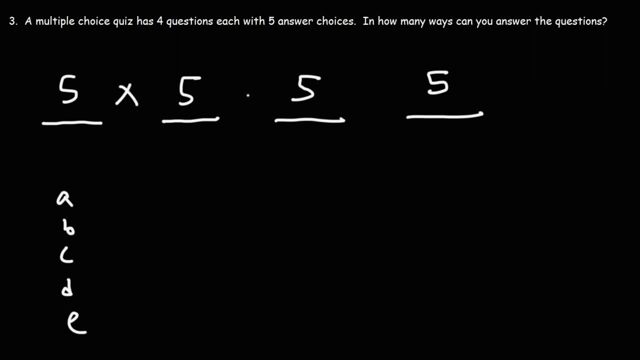 for the third and the fourth question. So you have five possible outcomes for each event and you have four events. So this is going to be five to the fourth power, or five times five times five times five. Five times five is twenty-five and twenty-five.